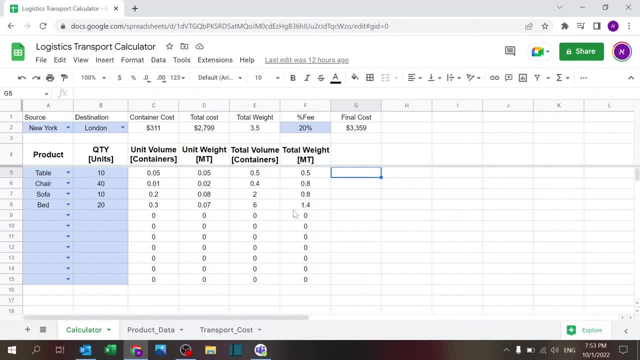 Okay, There we go. Alright, This is the first sheet, the main sheet. I just wanna tell you, if you guys enjoy the content that I'm publishing, please make sure to subscribe, like and share with your friends and colleagues to help this channel grow. 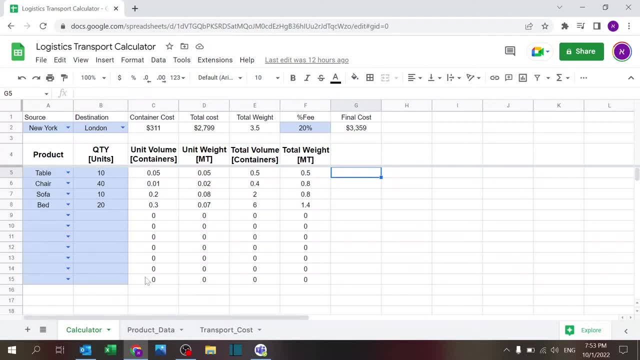 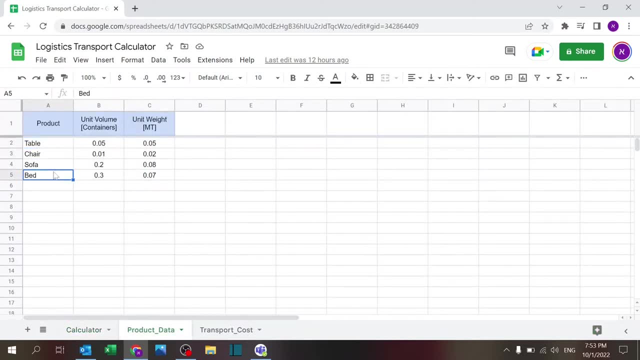 I would really appreciate that if you just squashed that button. Thank you. So Where some of the information is coming from, There is a sheet called Product Data where you define the product like table chair and sofa, And then you know of them. 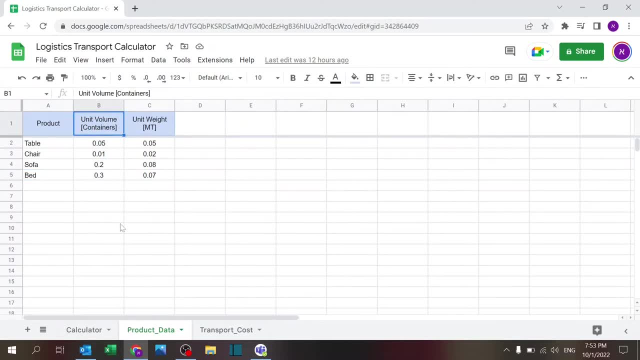 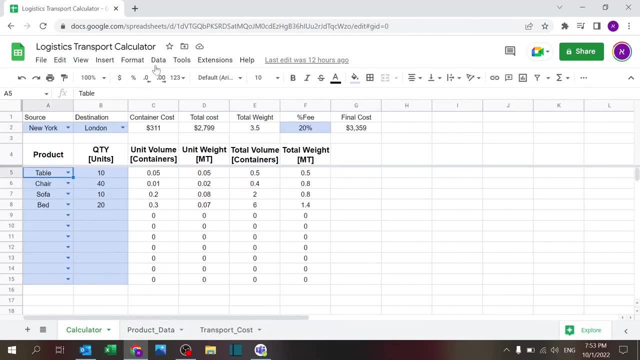 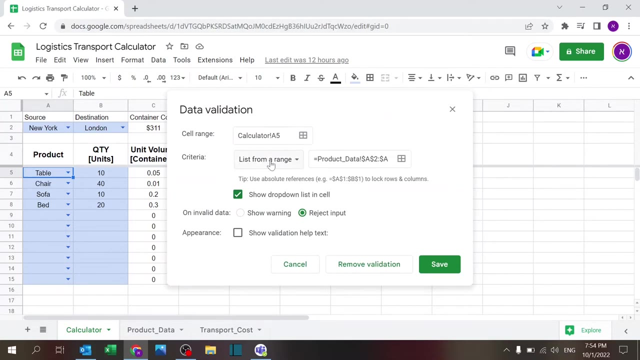 Down here you just click on it right the volume and containers and metric tons. then to use the drop-down. if you're not familiar with that, that's very simple. go to data, data validation and here you select list from. you know what? I'll just do it from the beginning. go to 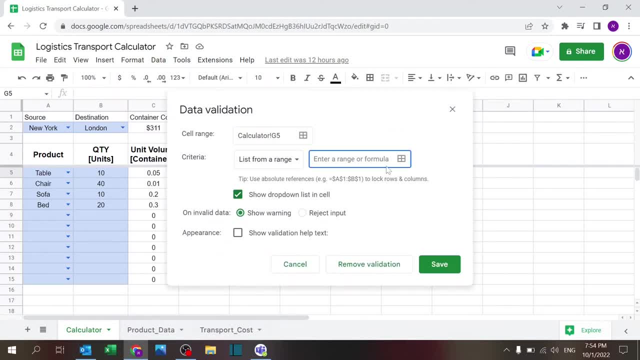 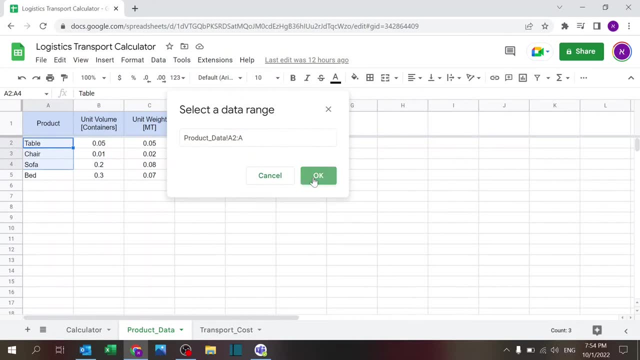 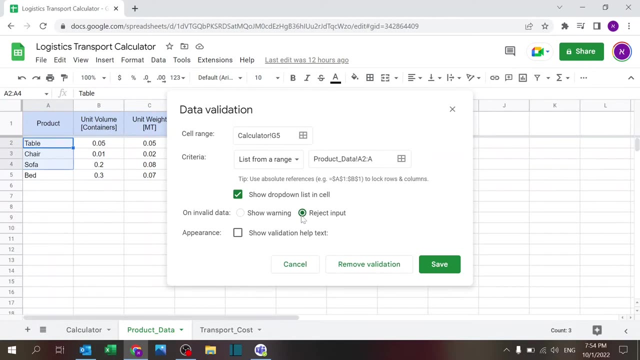 data data validation. it will look like this: you click over here on this and you just select the first one, and I just like to keep this blank and that would just give it everything that you have all the way down and reject input, as I don't want you to be able to input any other value. save and that's it. that's how. 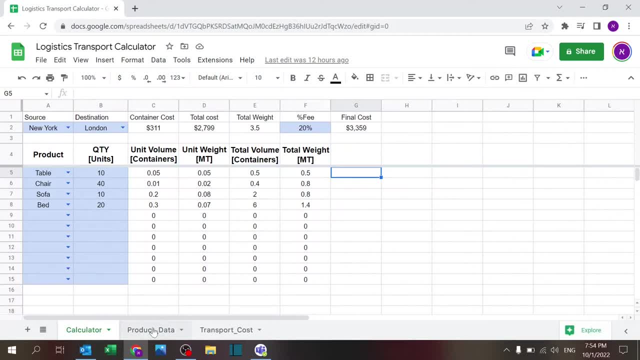 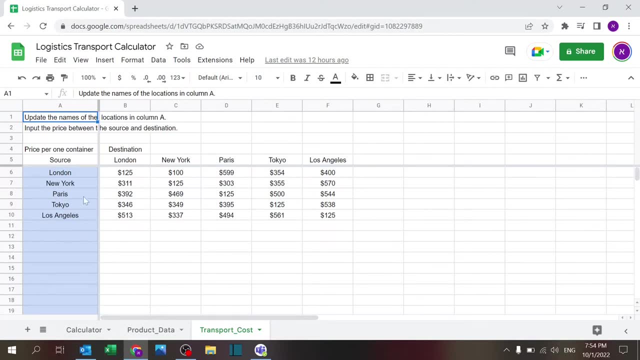 you do the drop-down list very easy, very simple. so that's the product data. transport cost is where you define the source and destination and the costs, and you'll notice that I only have one product and I only have one container. only highlighted this column because I'm using the transpose formula to give that. 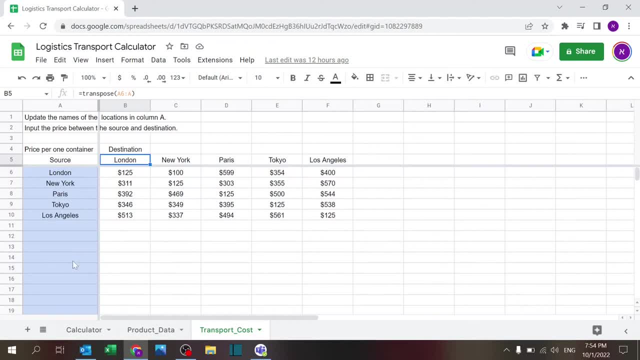 same names in the column and the row. so you have a source and destination and the logic here is that here you would put the. the cost to transport one container from here to here, so from Paris to Tokyo, is $500, but inside London it's 125 dollars and of course you can change that however you see fit. so these